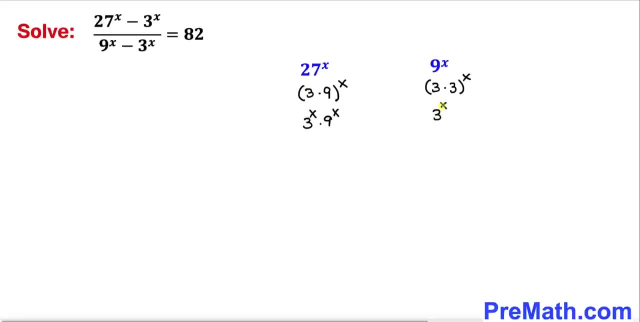 or this could also be written as: 3 power x times 3 power x. So therefore, this our original equation is going to become: now I'm going to replace this 27 power x by this. So therefore I can write this: 27 power x times 9 power x, minus 3 power x divided. by now, I'm going to replace this: 9 power x. 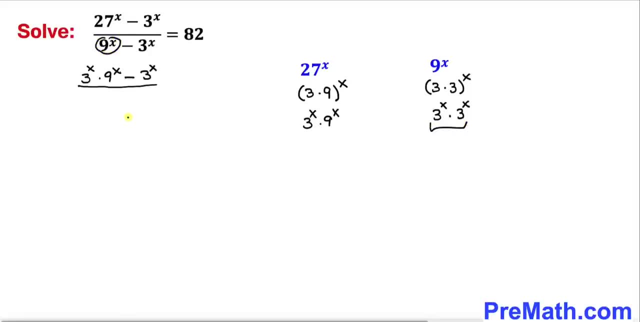 by this part. So I am going to write down: 3 power x times 3 power x minus 3 power x equals to 82 on the right hand side, So that 3 power x and this 3 power x is in common on the numerator, and likewise 3 power. 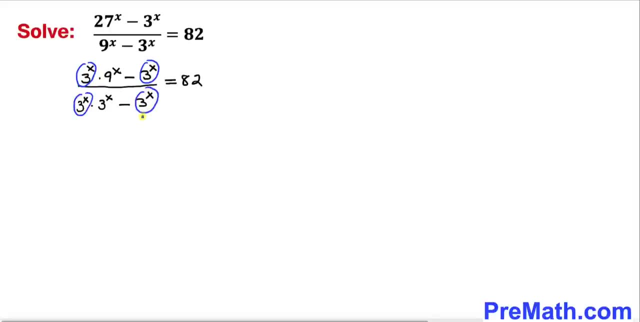 x and this 3 power x is in common in the denominator as well, So therefore I can factor out 3 power x on the top and inside the parenthesis is going to be 9 power x minus 1, divided by 3 power x times 3 power x. 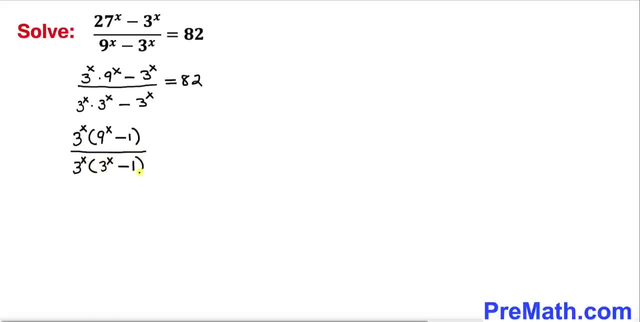 3 power x minus 1 equals to 82.. And now we can see this: 3 power x and 3 power x. they are gone. So we are ended up with 9 power x minus 1. divided by 3 power x minus 1 equals to 82.. Now let's focus. 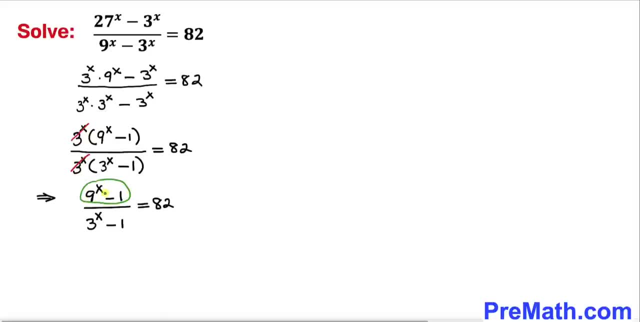 on this part in the numerator 9, power x minus 1.. And here I have copied it down and we can see this: 9 could be written as 3 times 3: power x minus 1. divided by 3, power x minus 1 equals to 82.. 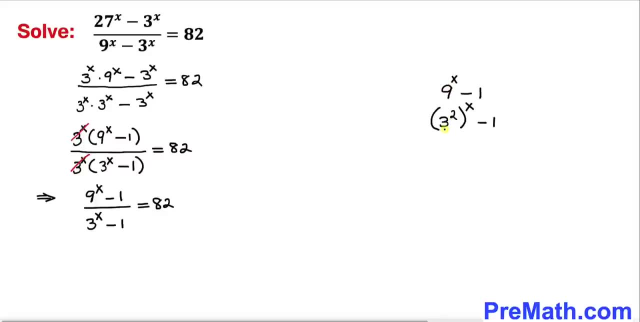 So how many times do they have to be written as 3 times 3 power x minus 1?? The answer is 3 power x and 3 power x minus 3 power x equals to 82. So therefore we can write 3 power 2 and whole power. 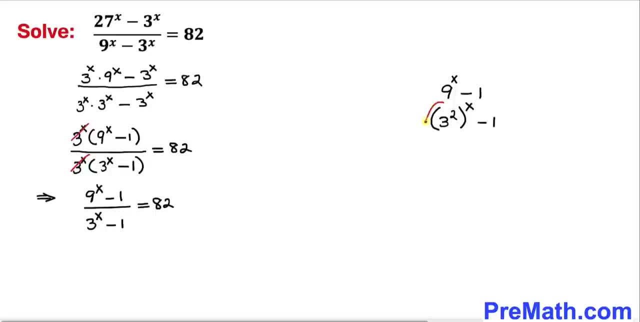 x minus 1.. And now let's focus on this part, only this one, And here I have copied it down. And now let's recall this power rule. according to this rule, We can write this one as a 3 power 2 x.